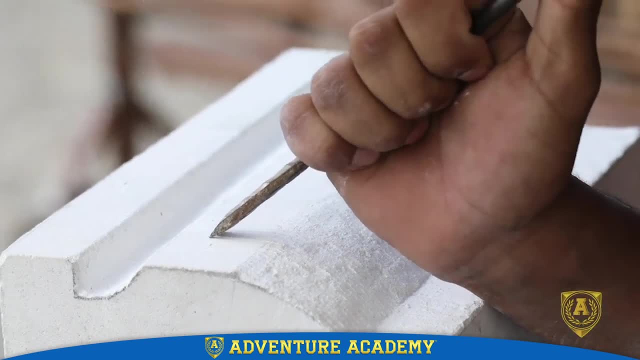 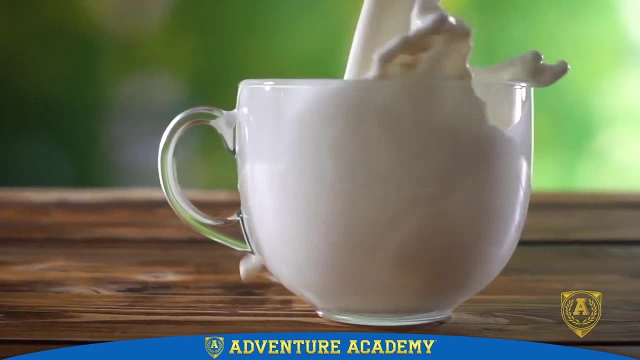 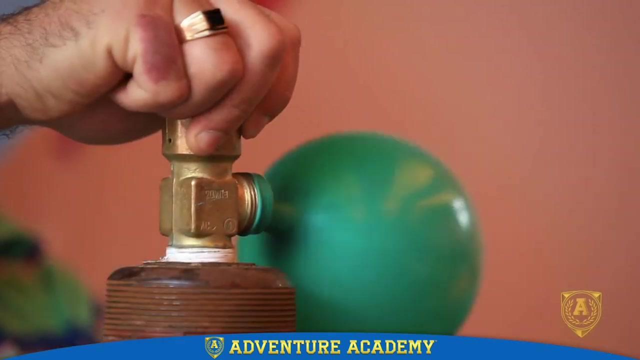 ice and stone are all examples of matter that hold their shapes as solids. When matter can flow easily and take the shape of its container, it is a liquid. Water, milk and honey are all liquids. Matter can also spread out to fill whatever space it's in, like air does. When matter acts like this, it's called a. 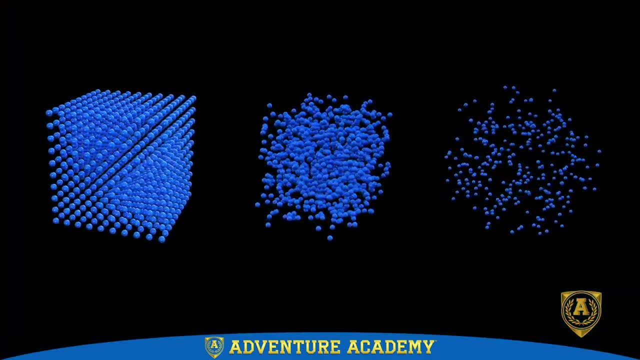 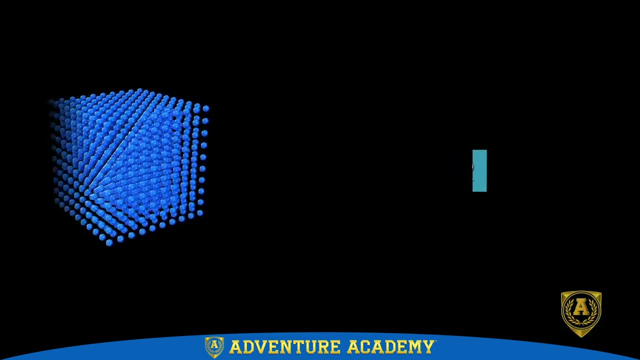 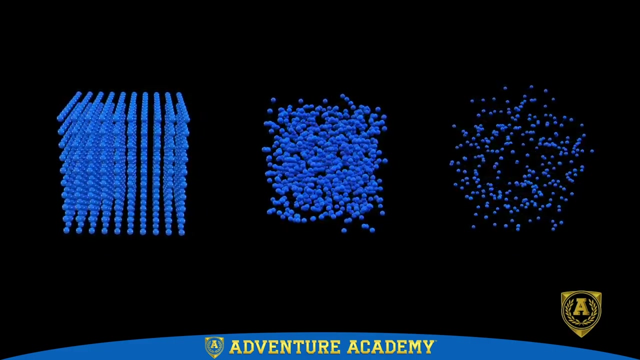 gas. These three forms of matter—solid, liquid and gas—are called states of matter. States of matter can change, going from solid to liquid and liquid to gas and back again. It all has to do with the arrangement of atoms and molecules. Atoms and molecules in a solid. 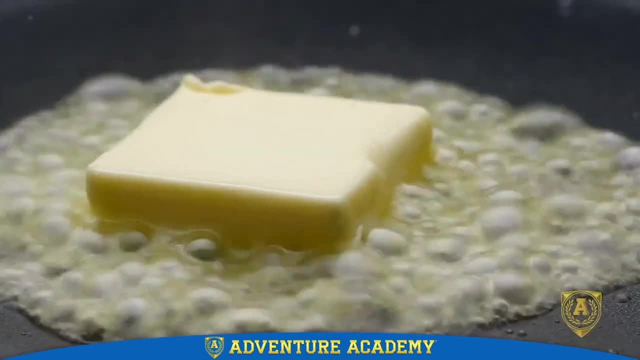 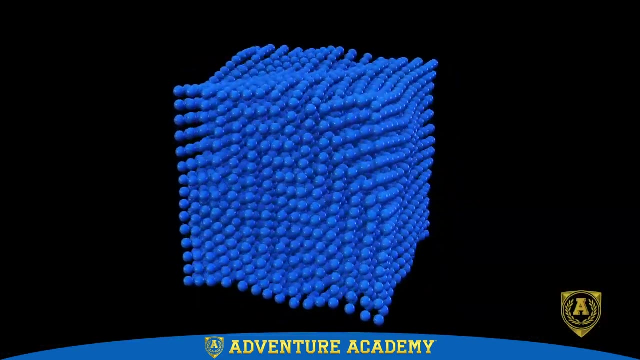 are locked tightly together, But when the right amount of heat energy is applied, those atoms and molecules get moving, Gaining energy from the heat. they begin to vibrate and move faster until all those atoms or molecules break away from each other and flow more. 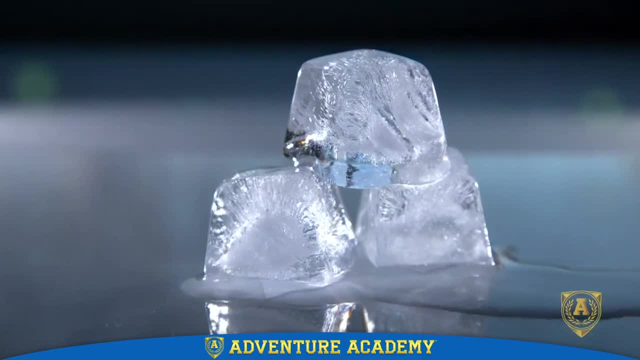 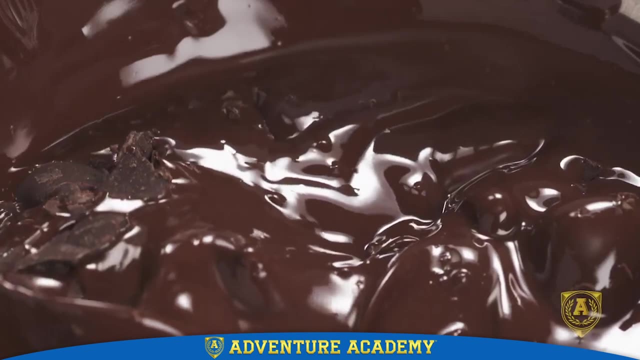 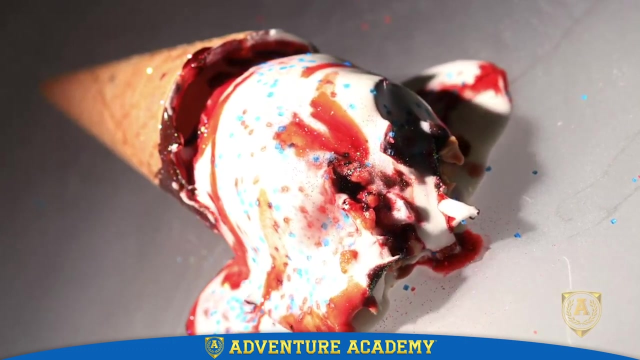 When something solid becomes a liquid, usually by the application of heat, we call it melting. You've observed this many times. When chocolate or butter or ice cream melts, we are seeing this in action And with enough heat energy, even very hard solids can be melted into a. 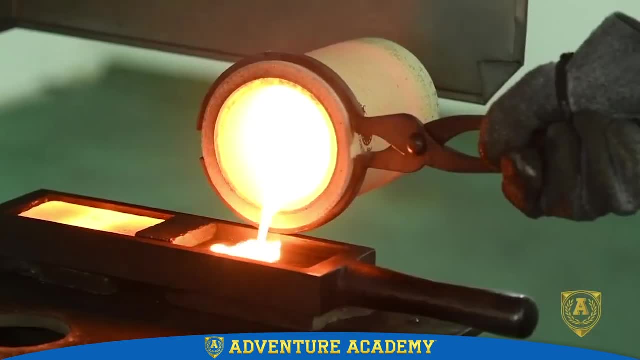 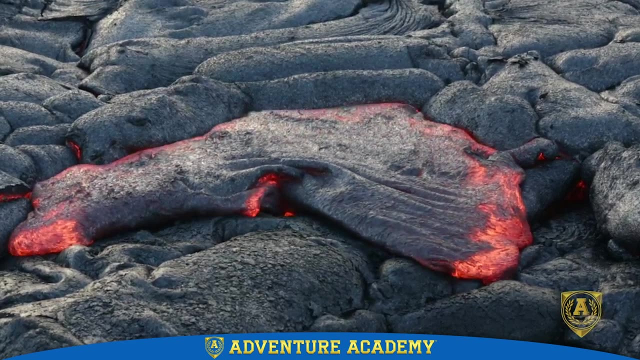 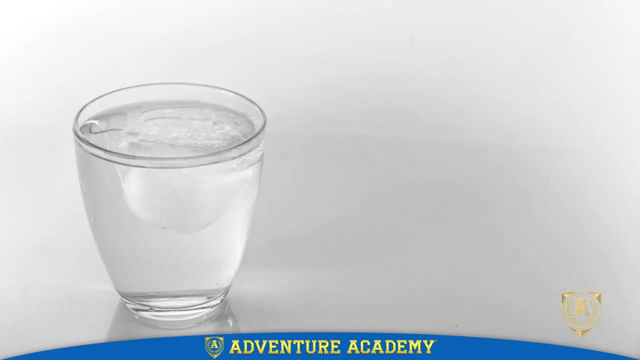 liquid state Metals like gold or aluminum can be poured into different shapes, Even certain kinds of rock, when heated enough, melt and begin to bubble and flow. The opposite action is also true When the liquid form of matter is cooled enough. it. 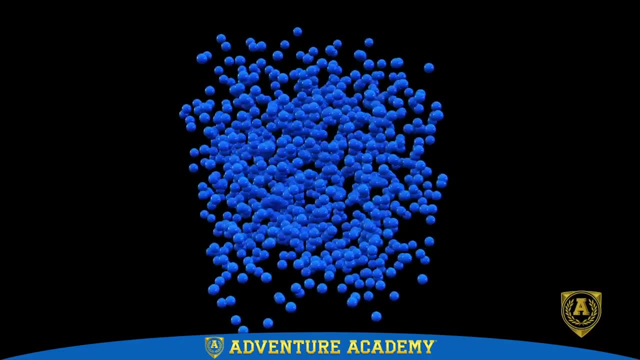 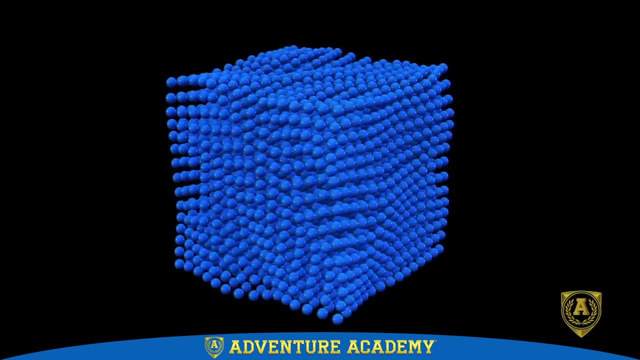 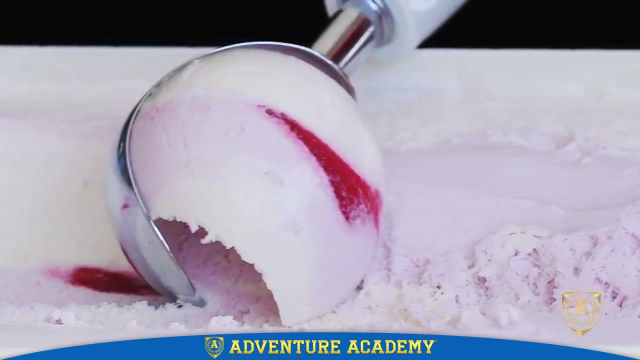 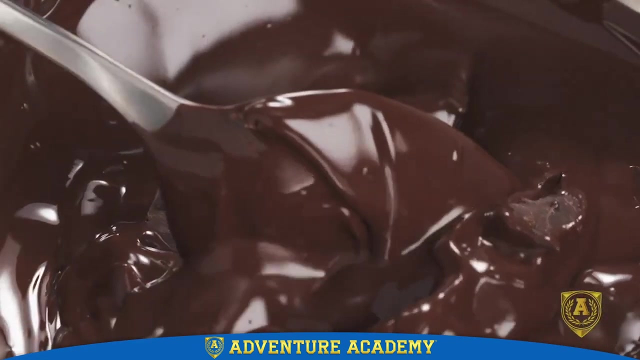 can freeze. Freezing happens when all of the atoms or molecules slow down and become locked together, changing the liquid into a solid. This is what's happening when water freezes into icicles Or fresh cream is frozen, Since solid matter holds its shape and liquid matter does not. many of our favorite things 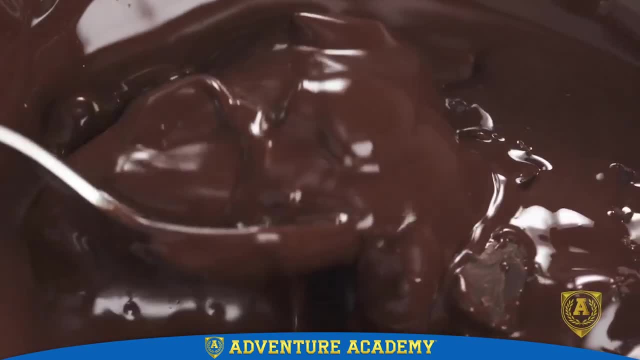 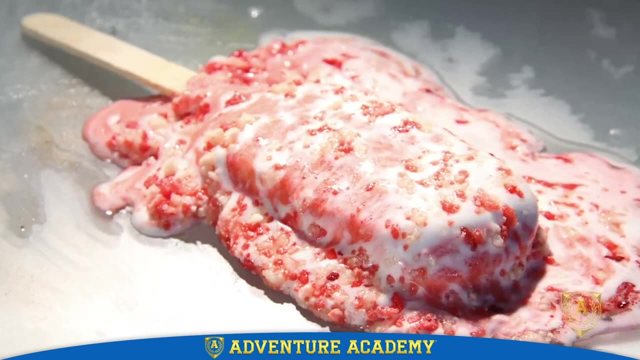 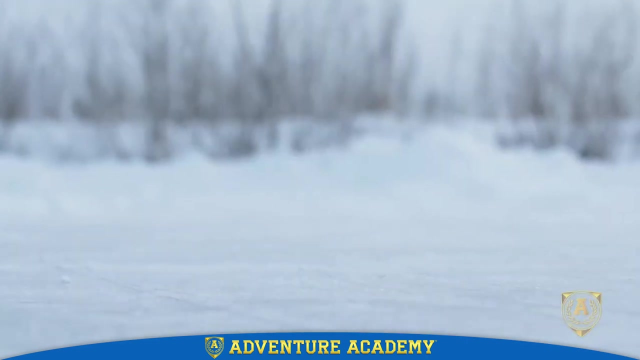 can be created by taking advantage of these changing states of matter, like chocolate candies and gold bars. So the next time your popsicle melts on the counter or you're enjoying ice skating on a frozen pond, think about the different states of matter all around you and how they make.